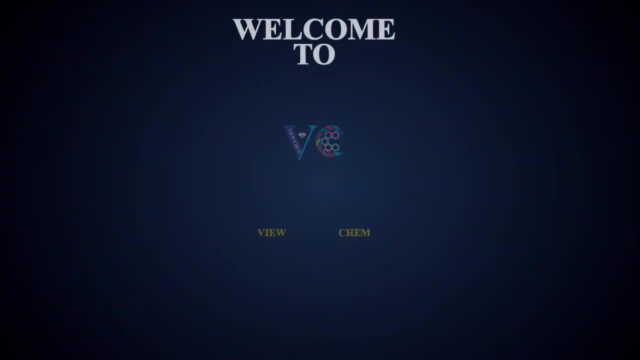 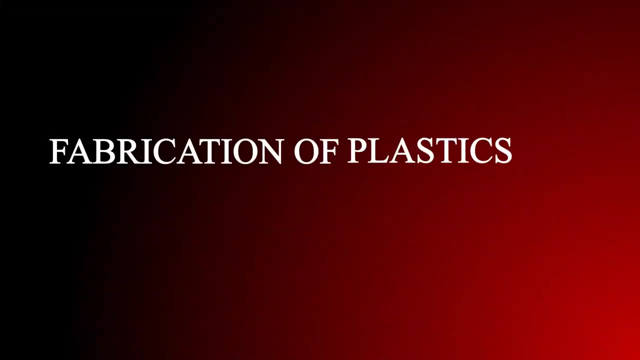 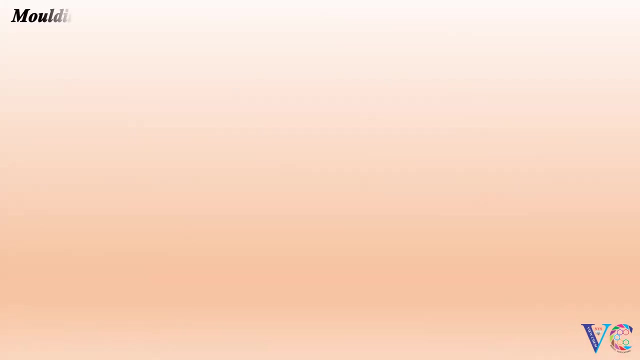 Welcome to VIEWCHEM, the Chemistry Animations Channel. Fabrication of Plastics or Molding of Plastics. Molding of Plastics: Molding of Plastics is carried out to obtain the desired shape. There are four major techniques by which plastics are molded. 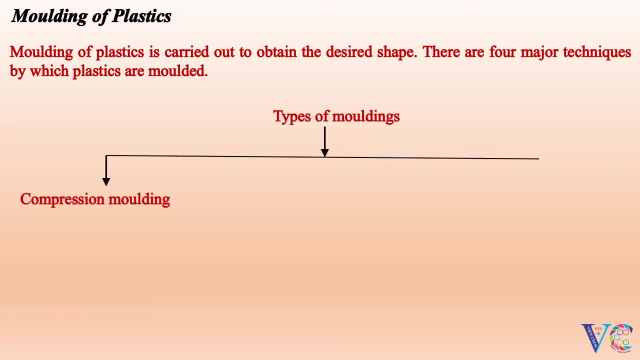 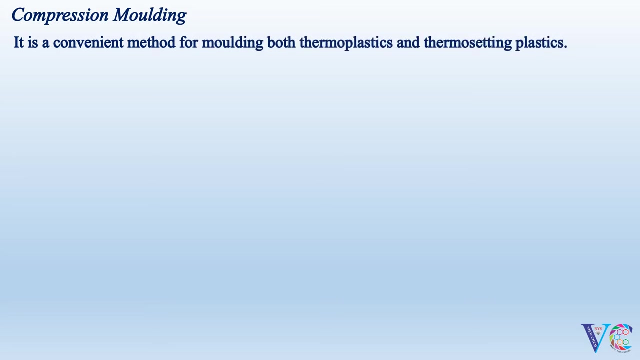 Types of Molding: Compression Molding: Injection Molding, Transfer Molding, Extrusion Molding- Compression Molding: It is a convenient method for molding both thermoplastic and plastic Plastics and Thermosetting Plastics. The plastic material to be molded is filled into the lower part of the molding tool. 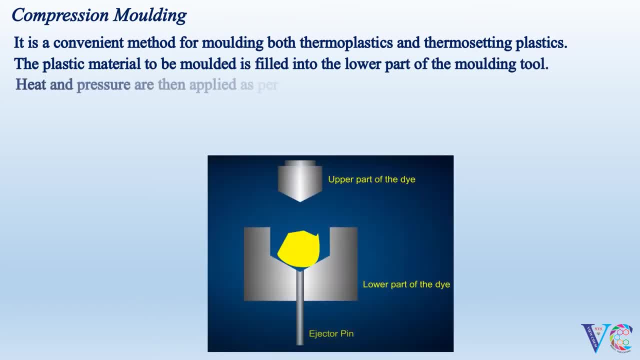 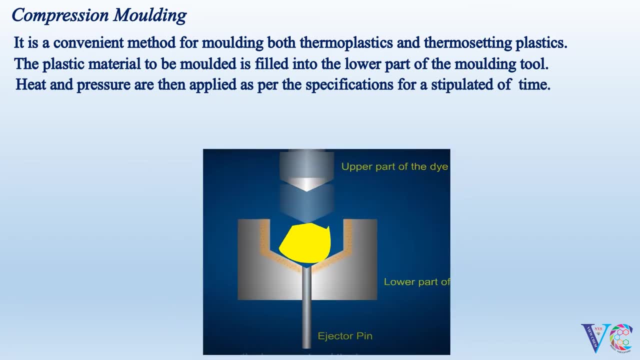 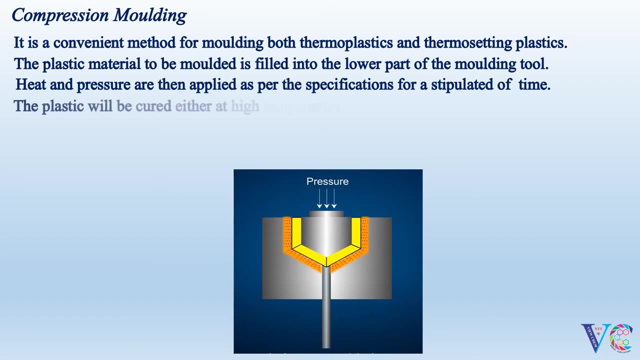 Heat and pressure are then applied as per the specifications for a stipulated period of time. Molding of Plastics: The plastic will be cured either at high temperature for thermosetting plastics or at low temperature for thermoplastics. Molding of Plastic: The cured plastic is taken out of the molding tool for further processing. 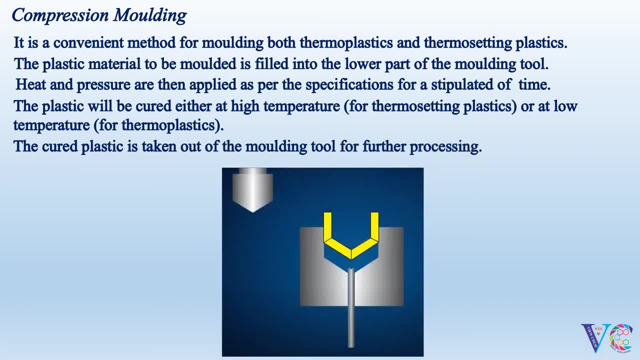 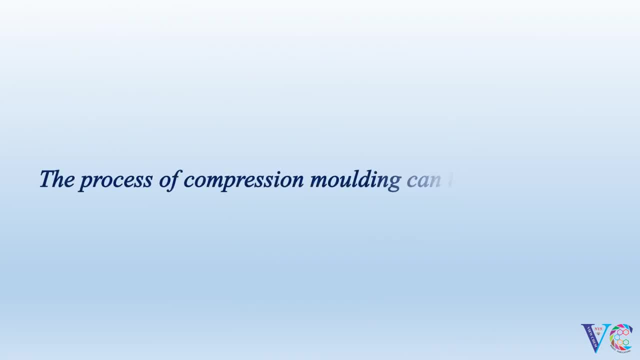 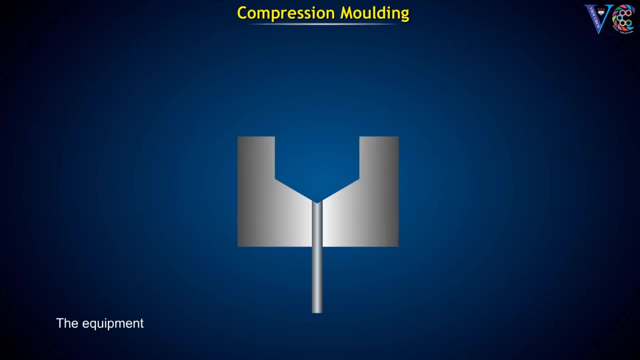 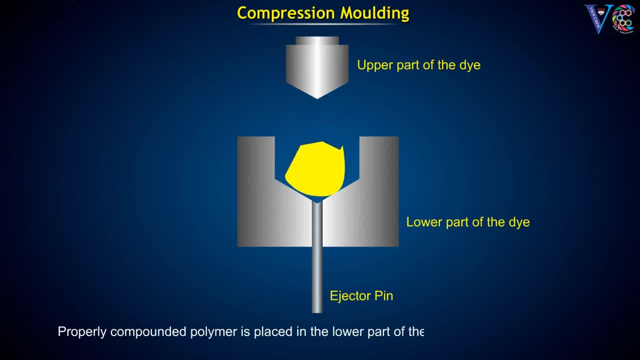 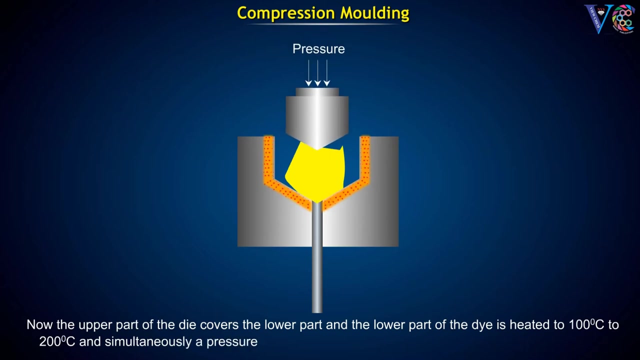 Properly compounded polymer is placed in the lower part of the die in the designated area. Now the upper part of the die covers the lower part and the lower part of the die is heated to 100°C to 200°C and simultaneously a pressure of 100 to 500 kg per cm2 is applied on the upper part of the die. 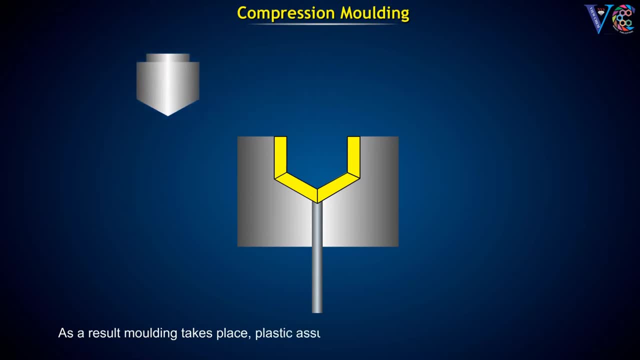 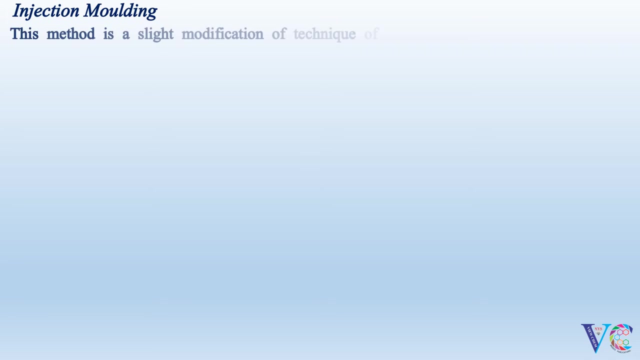 As a result, molding takes place, plastic assumes the desired shape and then is taken out. In this manner, the process continues. Injection molding: This method is a slight modification of the technique of compression molding. It is more advantageous because compression molding is a batch process, while injection molding is a continuous process. 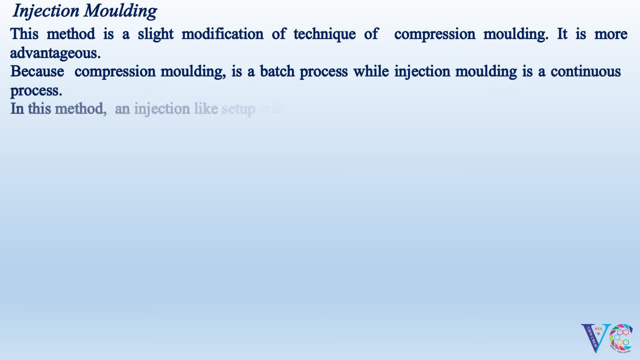 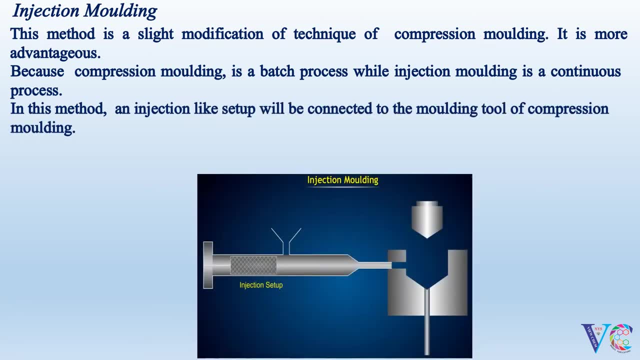 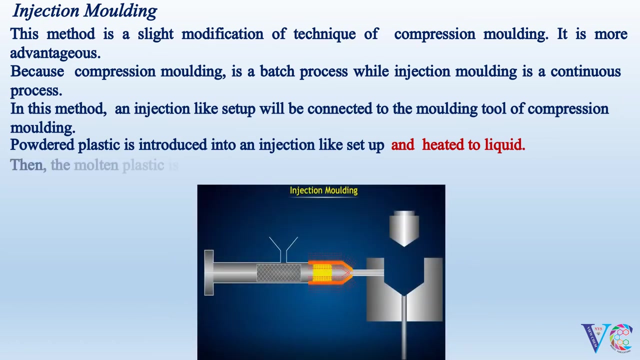 In this method, an injection-like setup will be connected to the molding tool of compression molding Packaging. Powdered plastic is introduced into an injection-like setup and heated to liquid. Then the molten plastic is pushed into compression molding tool with help of a piston. 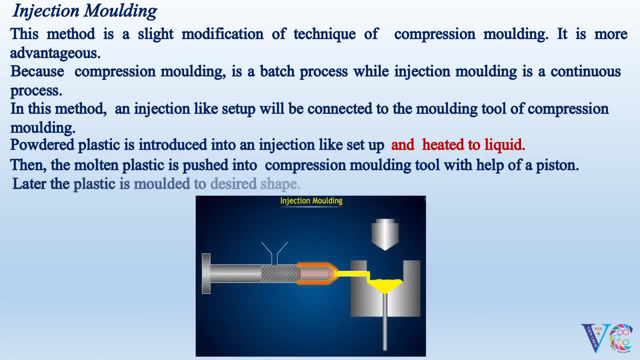 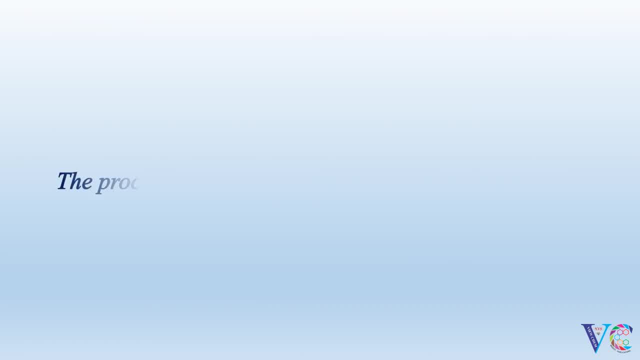 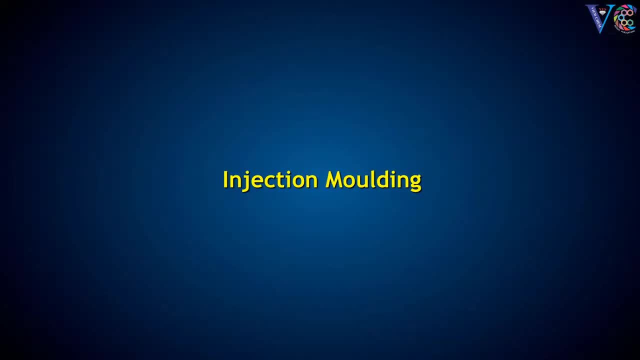 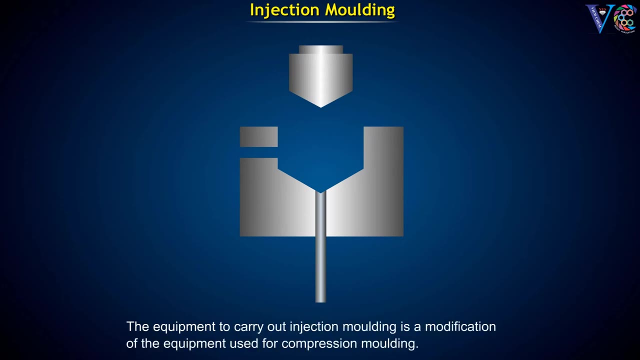 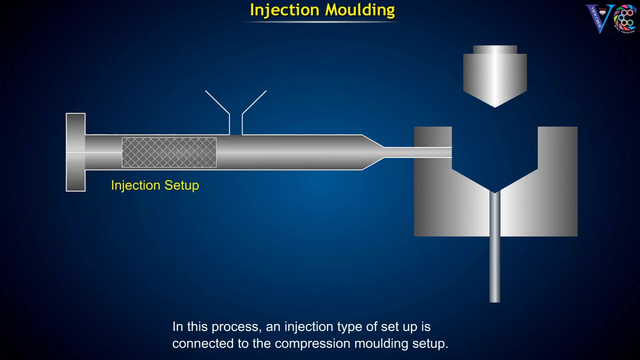 Later the plastic is molded to desired shape. Injection molding: The process of injection molding can be visualized as Injection molding. The equipment to carry out injection molding is a modification of the equipment used for compression molding. In this process, an injection type of setup is connected to the compression molding setup. 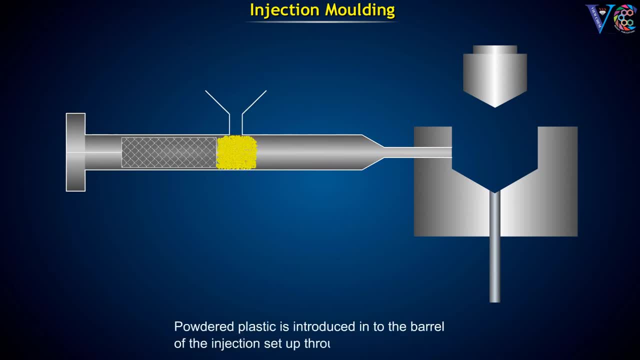 Powdered plastic is introduced into the barrel of the injection setup. The piston is pushed such that the powdered plastic moves forward where it is heated with the help of heating coils. As a result, the powdered plastic melts and further pushed into the mold. Now compression of the liquid plastic takes place to give the article of the desired shape. 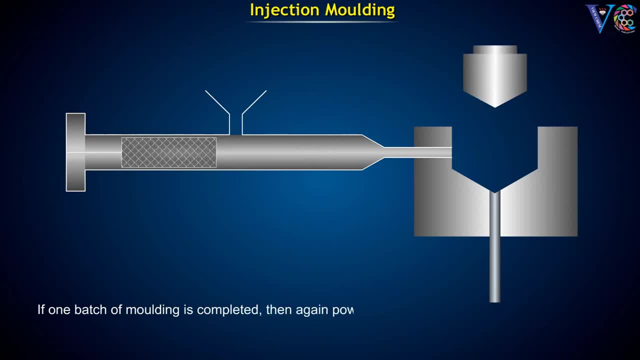 If one batch of molding is completed, then again powdered plastic is fed into the setup through hopper, pushed forward with the help of the piston, heated with heating coils. The liquid plastic is filled into the mold and gets molded, as in the case of compression molding. 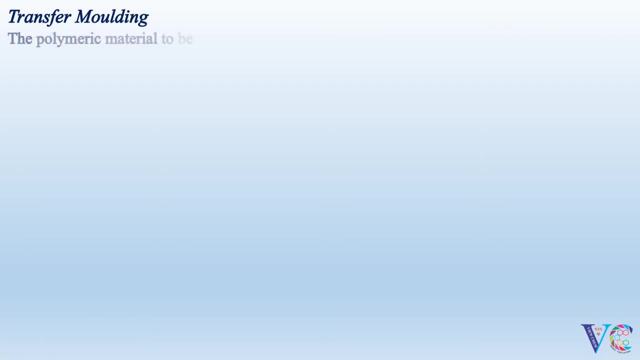 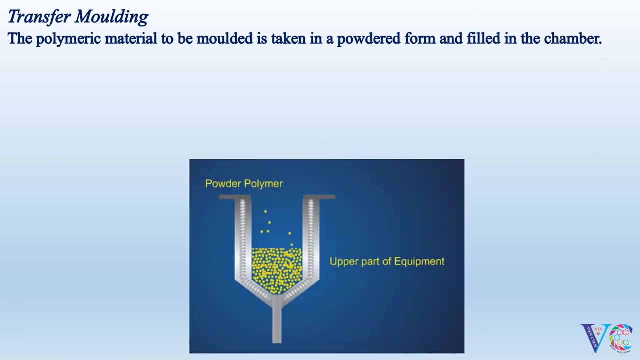 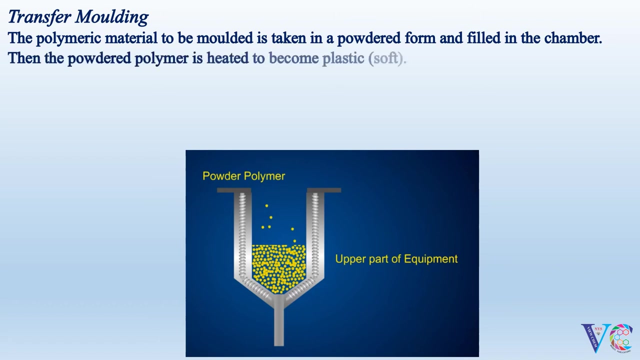 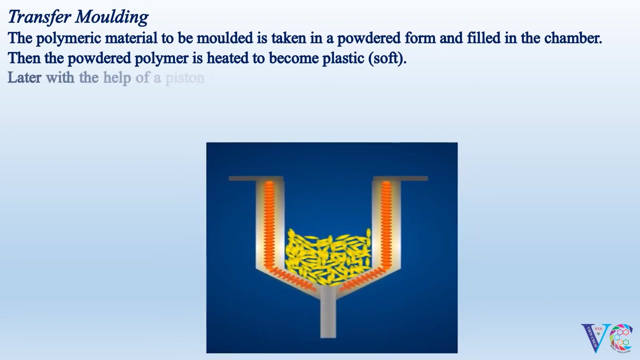 Transfer molding. The polymeric material to be molded is taken in a powdered form and filled in the chamber. The polymer videos powdered in tours of a AOA. Then the powdered polymer through the central pavedissa, anatomist wowd, is heated to become plastic, that is. 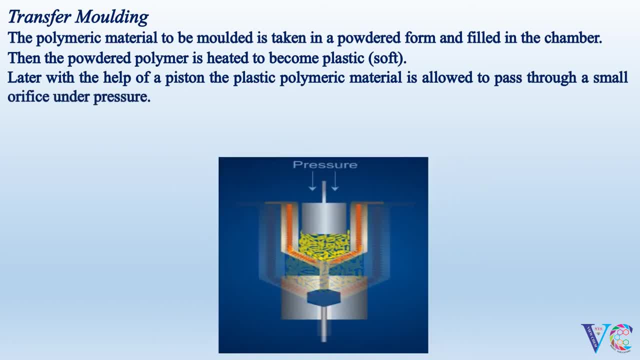 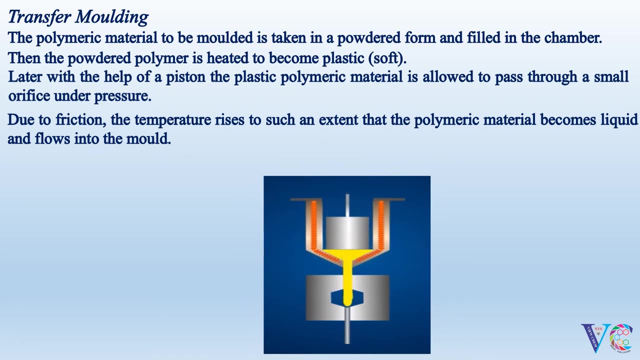 soft. Later, with the help of a piston, the plastic polymeric material is allowed to pass through a small orifice under pressure, to the extent that the polymeric material becomes liquid and flows into the mold. After curing under appropriate conditions, the molded plastic. 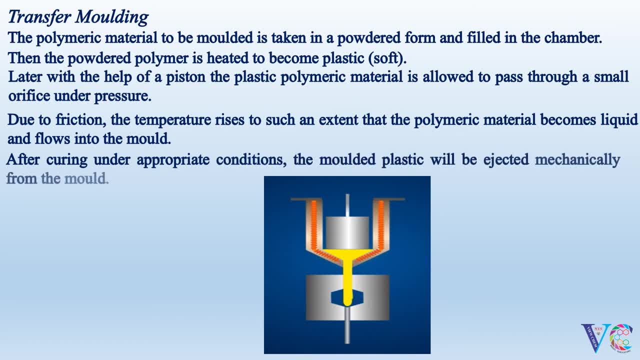 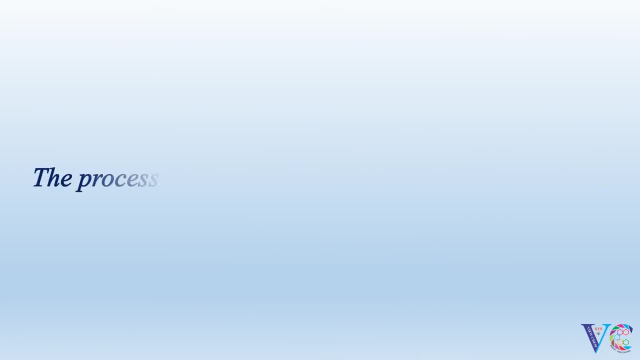 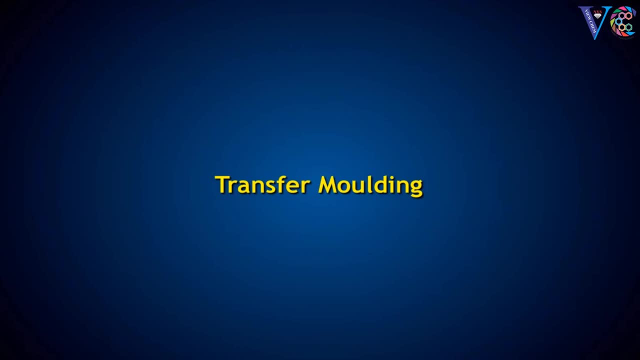 will be ejected mechanically from the mold. The process of transfer molding can be visualized as Transfer molding. In the transfer molding into the upper part of the equipment, properly compounded powdered polymer is introduced. In the next step, the powdered plastic is heated moderately such that it becomes plastic. 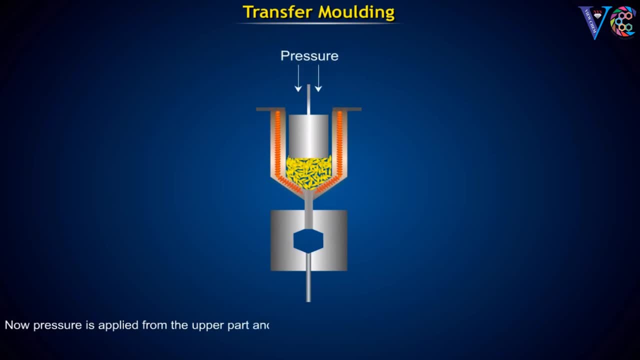 Now pressure is applied from the upper part and the polymer is forced to pass into the lower part of the mold. At this juncture, the polymer experiences more heat due to the pressure developed at the aperture, hence liquefies the liquid polymer passes into the lower part of the mold. 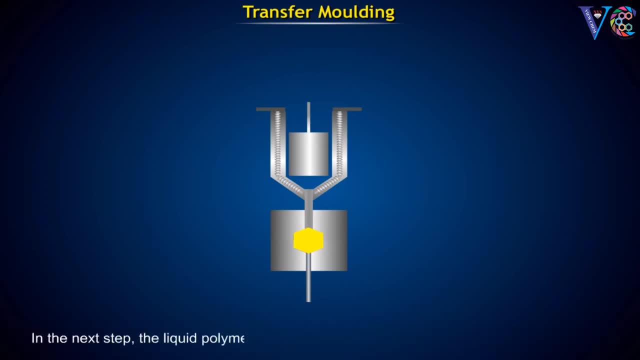 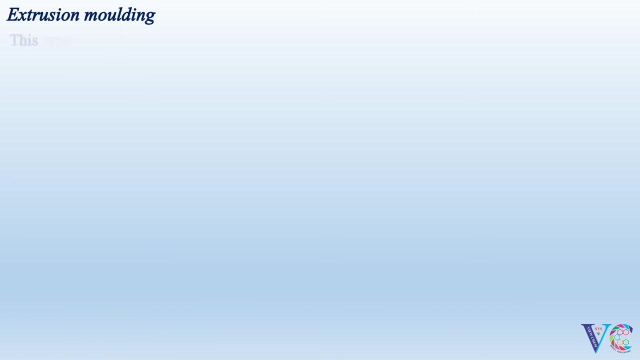 In the next step, the liquid polymer is heated to the curing temperature, then the molded polymer of desired shape is obtained and then taken out of the mold with the help of an ejector pin Extrusion molding. This type of molding is used in the preparation of continuous molds with uniform cross-section.